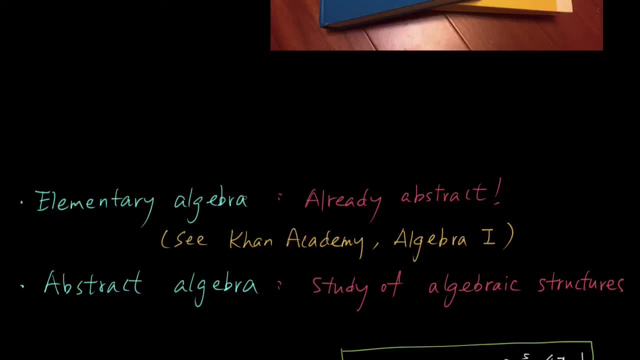 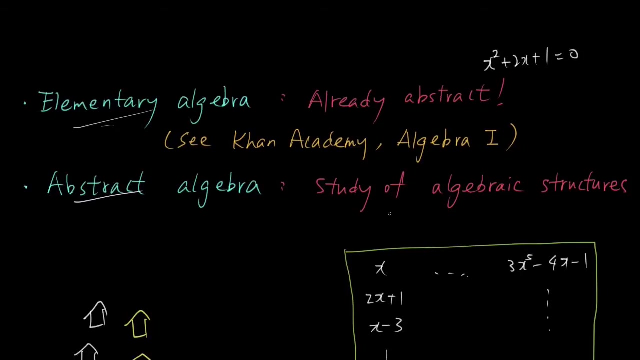 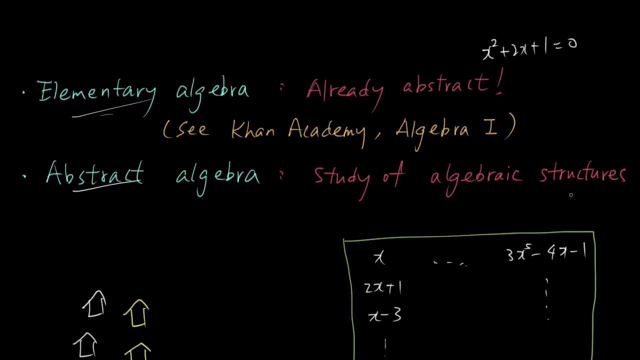 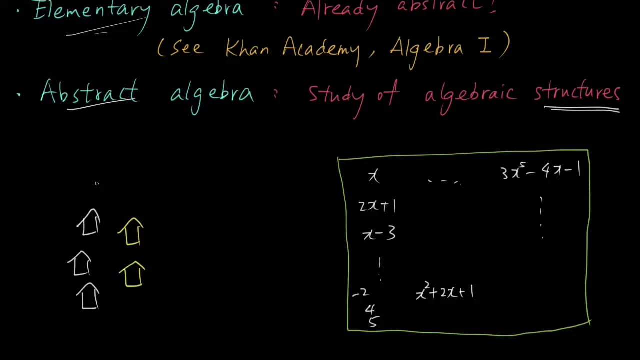 And if you've studied algebra before, you know that it is already pretty abstract, right? We study things like polynomial equations, like x squared plus 2x plus 1, let's say, equals 0, and that is an abstraction. In fact, Sal on Khan Academy also talked about this abstractness and beauty of algebra, so I highly recommend having a look at that. It's in the Algebra 1 section. So that is elementary algebra. And what about abstract algebra? Well, generally speaking, abstract algebra is the study of algebraic structures. So structure is the key word here. And for a mental image of what that means, let's imagine something concrete, like a village, okay? So, here is my village, with five poorly drawn houses or sometimes we may be interested in a single villager inside the village and what he or she likes or does but other times we might want to know things about the entire village so what does this group of people do and how do they interact how can we describe the village itself so we might say things like this this village is next to some body of water maybe a coast an ocean and most people fish for a living so we might say that this is a fisherman's village and sometimes knowing about the village can 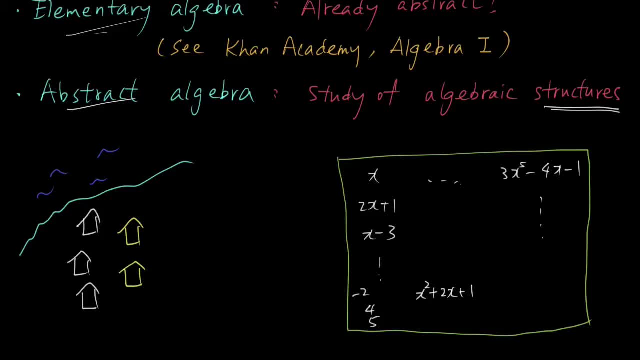 tell us us and can tell us things about individual say this boy out from coming out from the village can't draw a person so this boy from the village we might say that because he or she likes the village so we might say that because he is from the fisherman's village he might be a good swimmer in the real world we 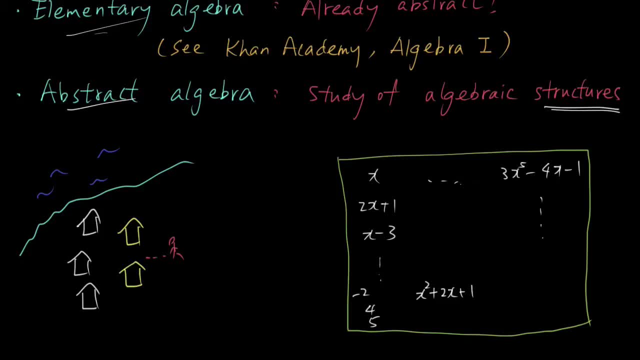 probably don't want to over generalize too much but that's kind of the idea right so moving back to the math world here and here on the right I have a box that represents an algebraic structure the box has a bunch of stuff inside much like there are people living inside a village so that's the parallel and what is in the middle of the village and what is in the middle of the village is a 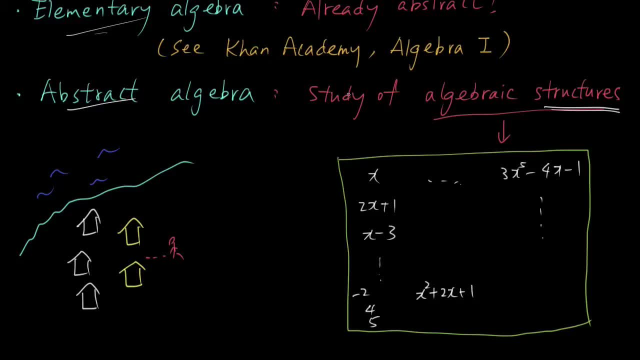 place in the box well I decided to skip the boring examples and put some interesting things in there so that is polynomials these are polynomials and I have a bunch of them loosely placed in the box but to have a structure that is not enough we also need to know how these things relate or how they interact just like how people in the village interact so for this example here I'm gonna say well now things in the box can 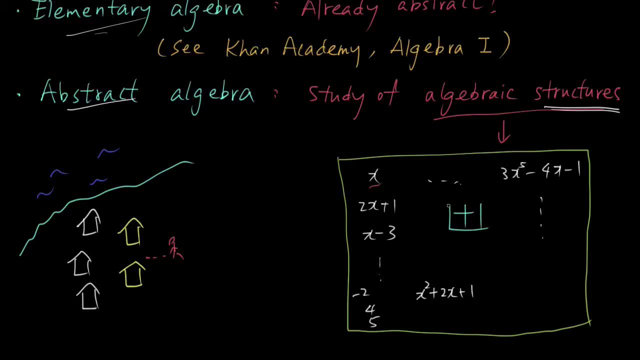 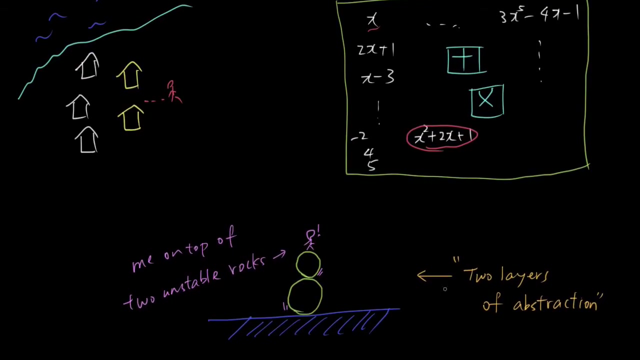 interact by addition that is I can add any two polynomials together and get a new one or I can do multiplication all right I can multiply two polynomials and get a new one so we have a collection of things and ways for them to interact and that is the basic model of what an abstract excuse me an algebraic structure is so this is roughly speaking the definition of an abstract structure the kind of object we study in abstract algebra and as you can see we kind of have two layers of abstraction here right say this polynomial a polynomial is an abstract entity right and then we are putting them inside this this abstract box extra collection so yeah sometimes it gets kind of tricky I kind of like this picture here that's me on top of two unstable rocks that's the image I have so this begs the question how is this ever going to be useful to 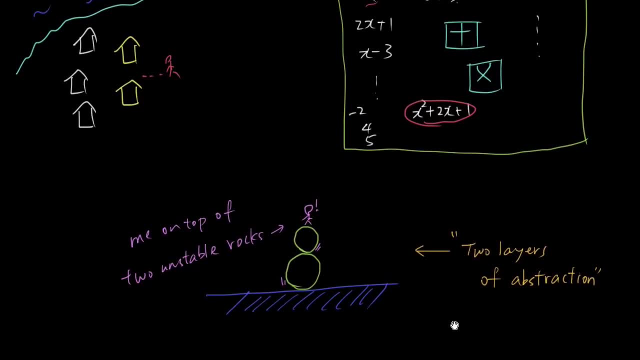 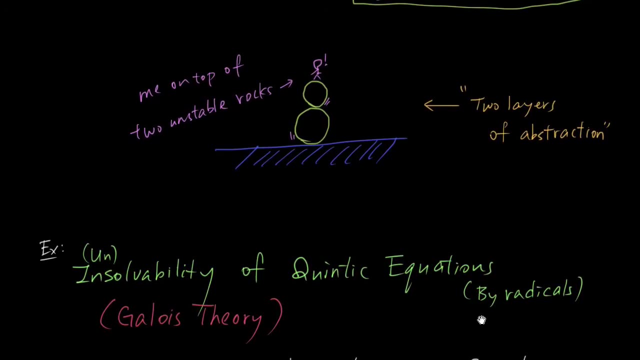 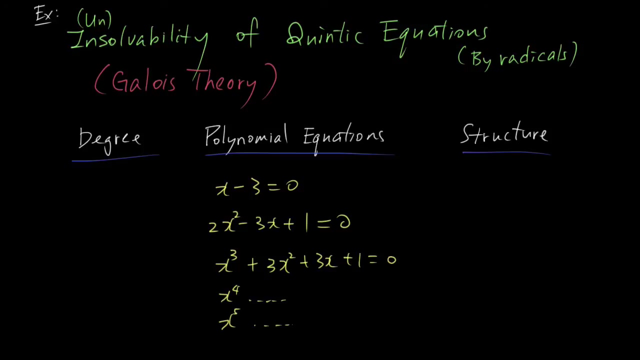 demonstrate its power I'm gonna try to describe a classic problem called the insolvability of quintic equations this is a topic called Galois theory Trivia Time Galois is a Frenchman back in the first half of eighteen hundreds he got into a duel at age twenty 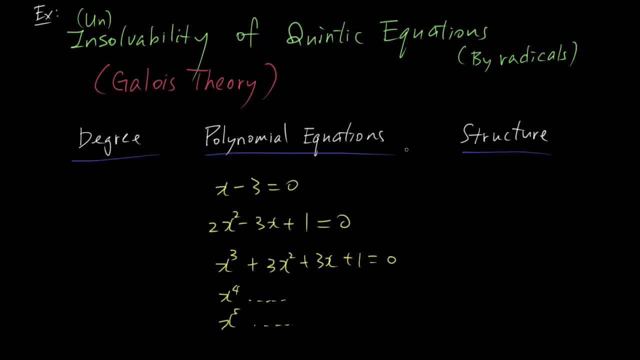 and I'm pretty crazy story but anyways the problem looks like this we have polynomial equations of different degrees linear of degree one quadratic of degree two degree three 3, 4, and 5, and so on. 5 is the quintic. 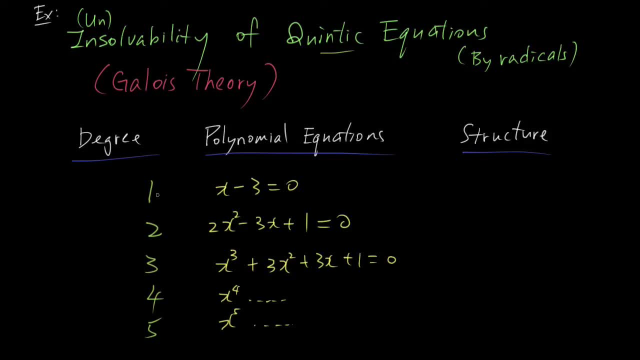 Now, what people found was that for equations of degree 1, 2, 3, and 4, they can all be solved in some pretty nice ways. And for example, the quadratic equation, this one here, can be solved with a formula. 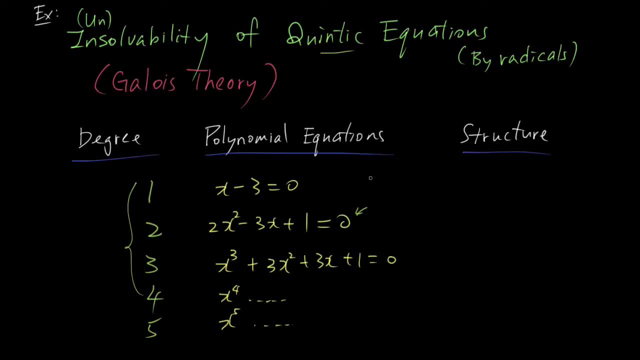 And a lot of us might be familiar with the formula. That looks like minus b plus or minus square root b squared minus 4ac over 2a, I believe. 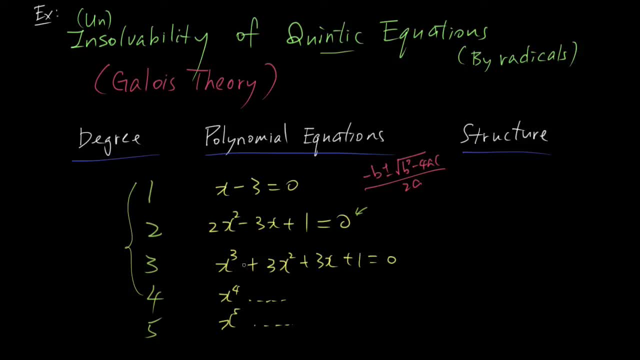 And there are similar formulas for degree 3 and degree 4 polynomials. But once you get to degree 5, though, suddenly you find equations that just can't be solved in a simple way like this. 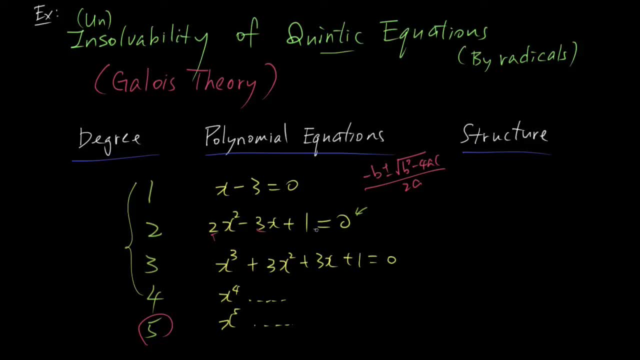 And by simple way, I mean you take the coefficients, and you add, subtract, multiply, divide, and take in roots, like this equation here. 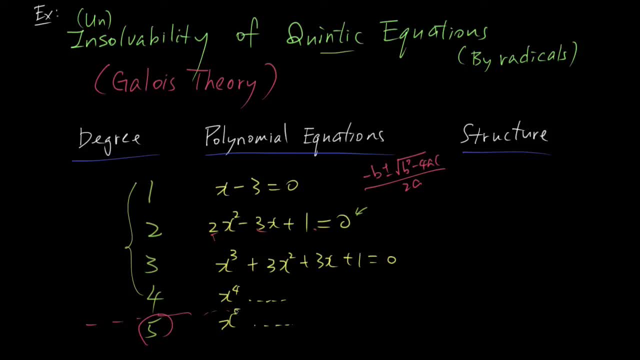 So for degree 5, this is like the dividing line here. Very strange. Why does that happen? 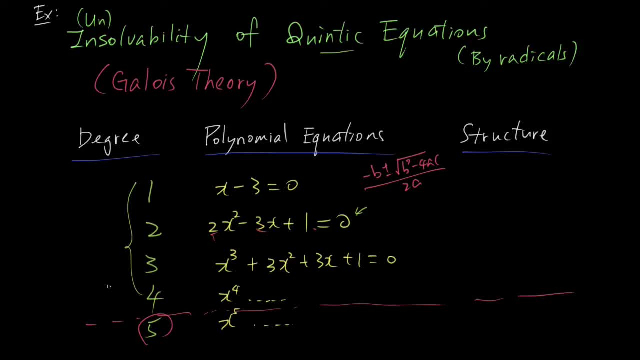 So imagine you are a physicist. You have to deal with high-degree equations, 5 or more. You're trying to solve your problem. And that could cause issues, right? You say you are having trouble. You're having trouble solving an equation. 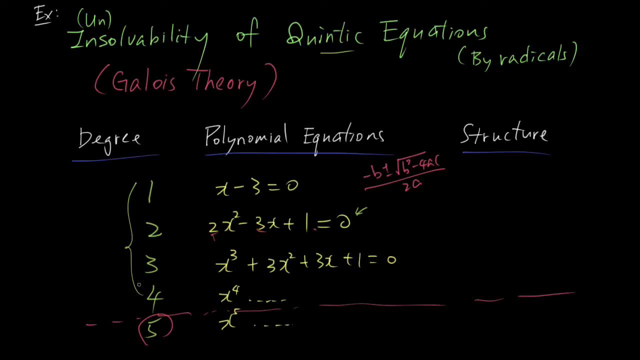 Does that mean you should try harder? Or is it just not solvable in the first place? That's kind of important to know. 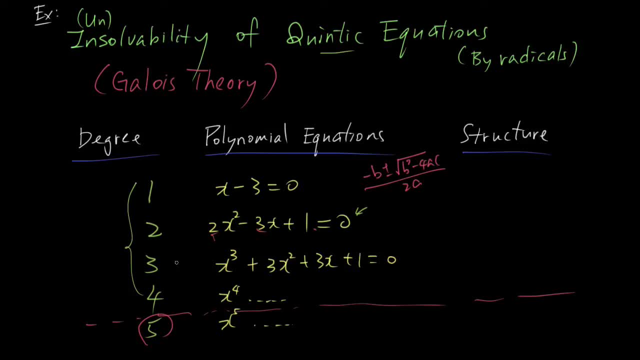 Fortunately, mathematicians answer the question for us using, yes, abstract algebra, of course. There's a kind of algebraic structure called the permutation groups. 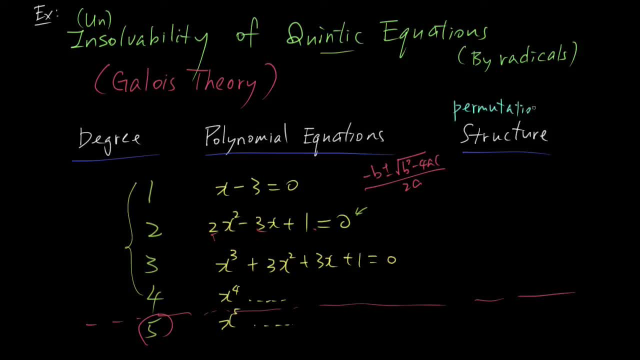 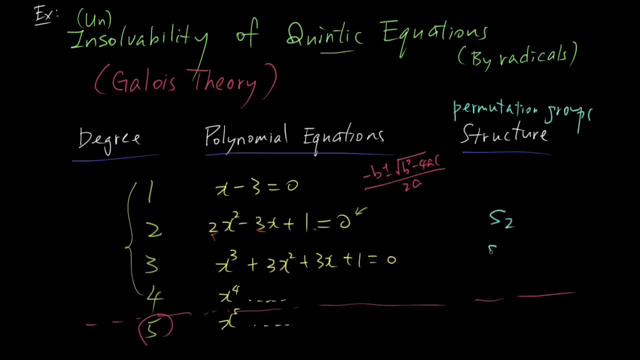 They're written like S2, S3, and so on, S4, S5. As it turns out, a degree 3 equation matches up with S3 in a very special way. 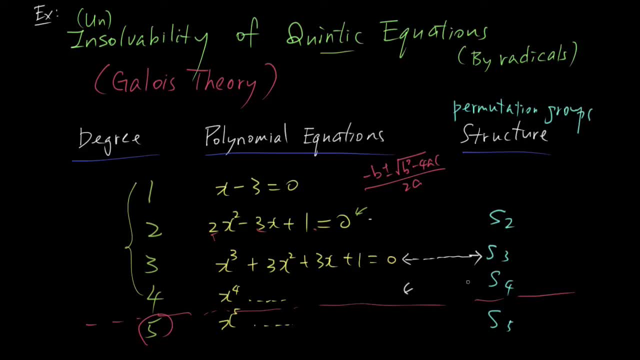 And degree 4 equation matches up with S4, and the trend continues. 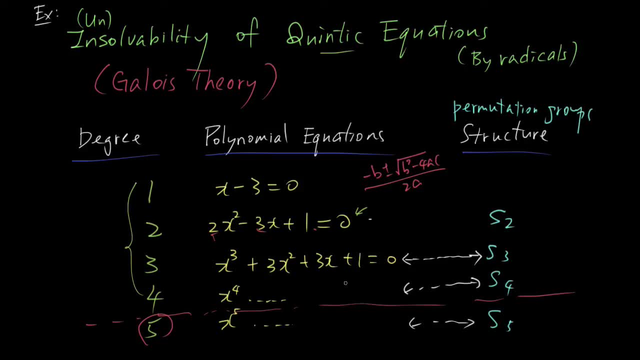 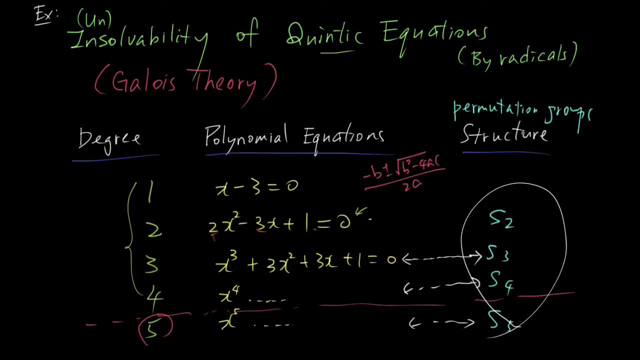 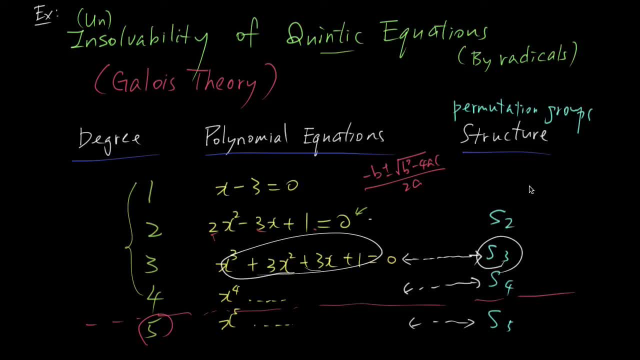 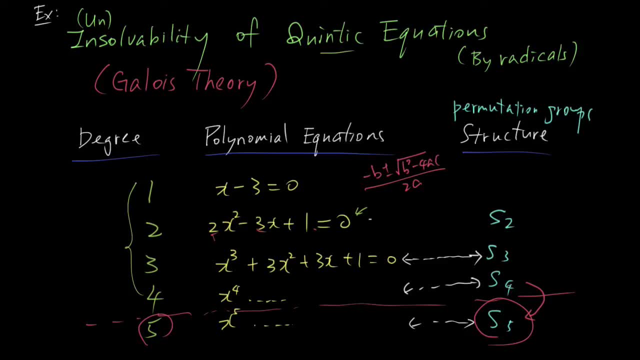 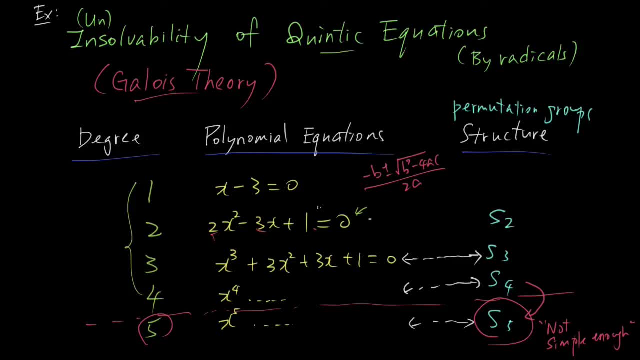